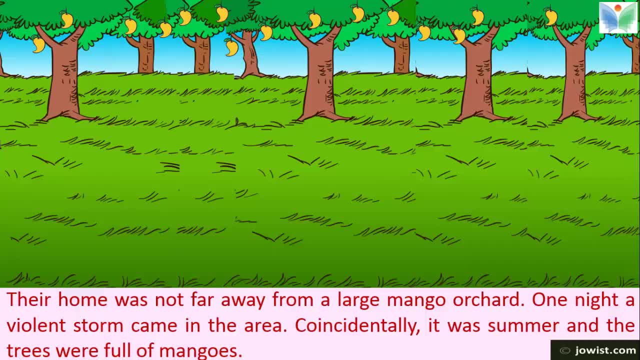 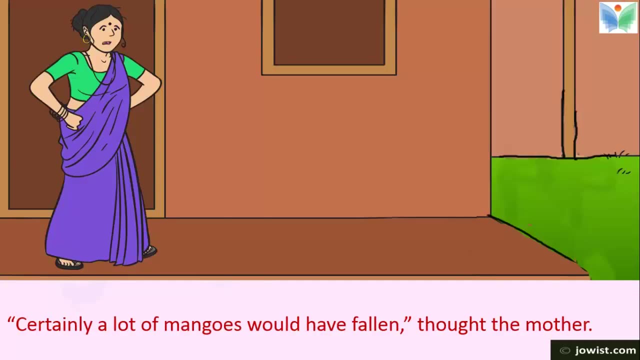 home was not far away from a large mango orchard. One night a violent storm came in the area. Coincidentally, it was summer and the trees were full of mangoes. Suddenly, a lot of mangoes would have fallen, thought the mother. 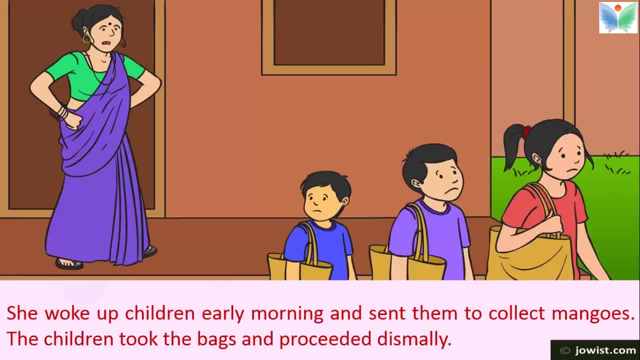 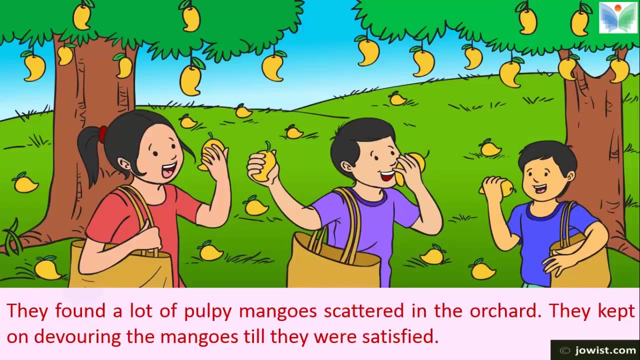 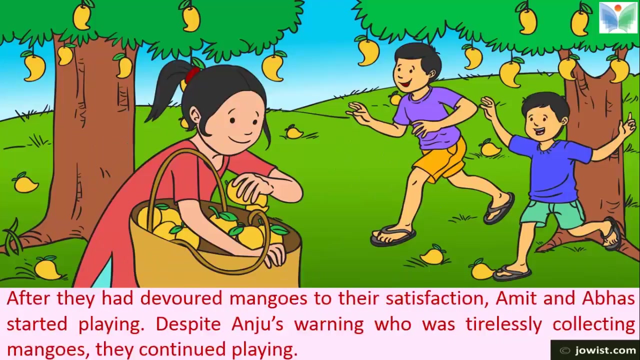 She woke up children early morning and sent them to collect mangoes. The children took the bags and proceeded dismally. They found a lot of bulky mangoes scattered in the orchard. They kept on devouring the mangoes till they were satisfied. After they had devoured mangoes, 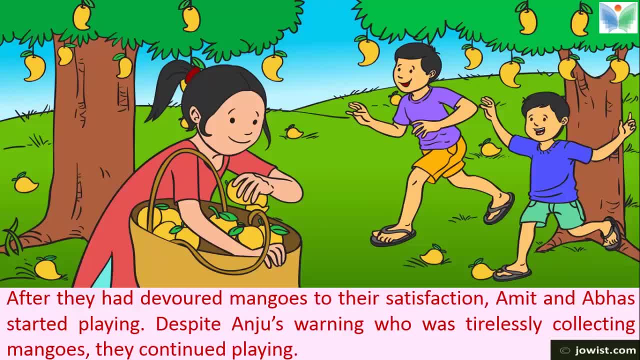 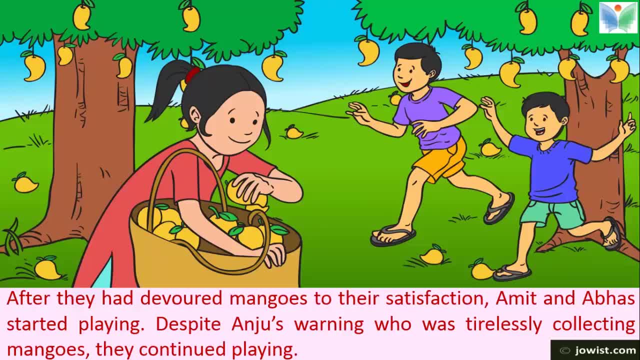 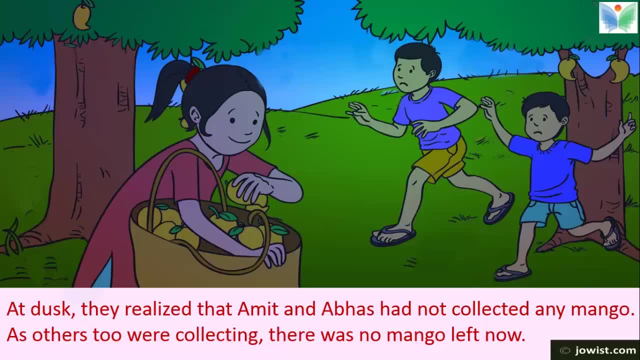 had no mangoes, They continued playing, Despite Anju's warning, who was tirelessly collecting mangoes. they continued playing. At dusk, they realized that Amit and Abhas had not collected any mangoes, As others too were collecting. there was no mango left, now Petrified of. 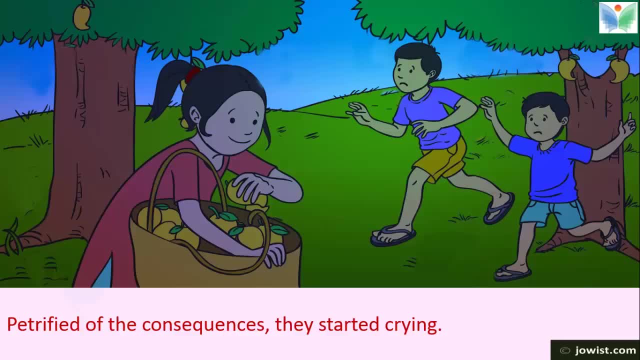 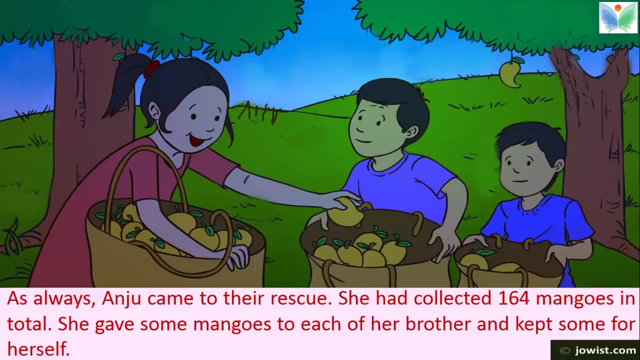 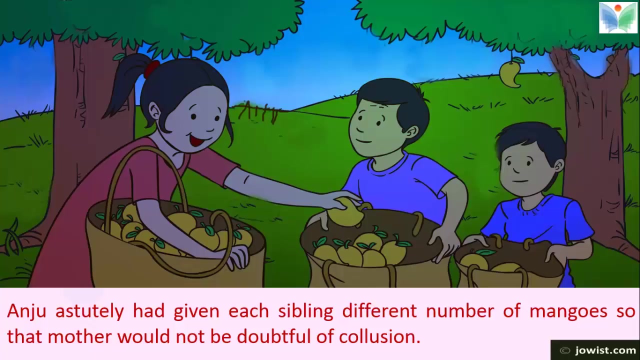 the consequences, they started crying. As always, the two of them were happy. Every Anju came to their rescue. She had collected 164 mangoes in total. She gave some mangoes to each of her brother and kept some for herself. Anju, astutely, had given each sibling different. 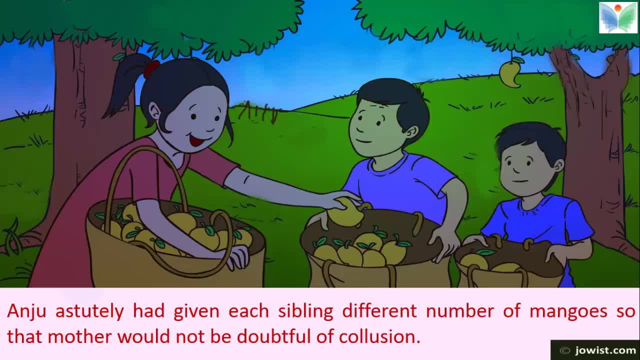 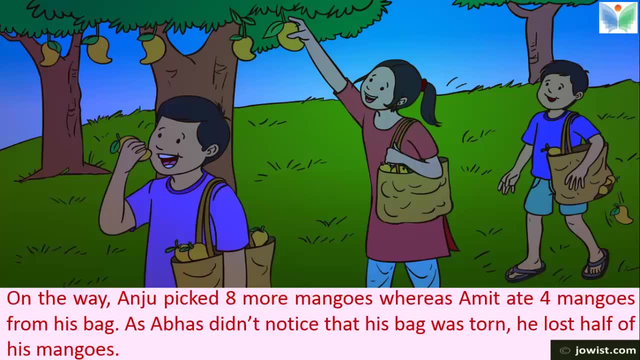 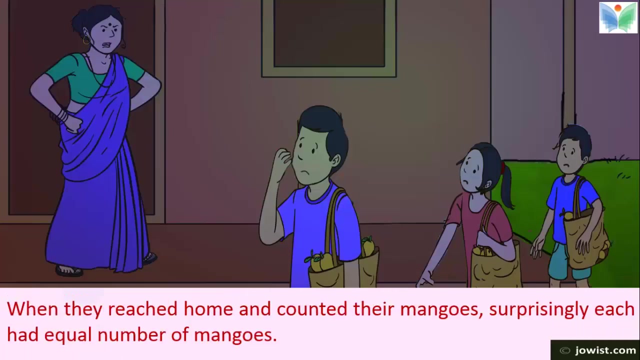 number of mangoes so that mother would not be doubtful of collusion On the way, Anju picked 8 more mangoes, whereas Amit ate 4 mangoes from his bag. As Abhas didn't notice that his bag was torn, he lost half of his mangoes When they reached home and counted. 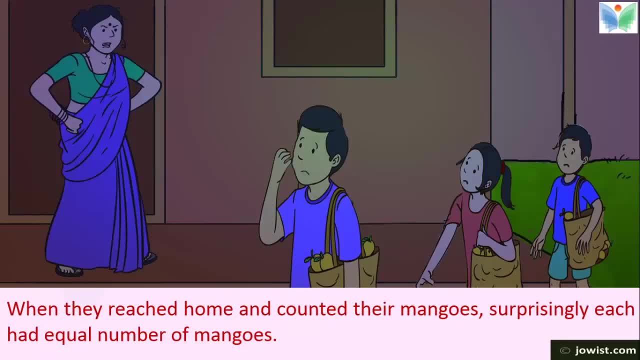 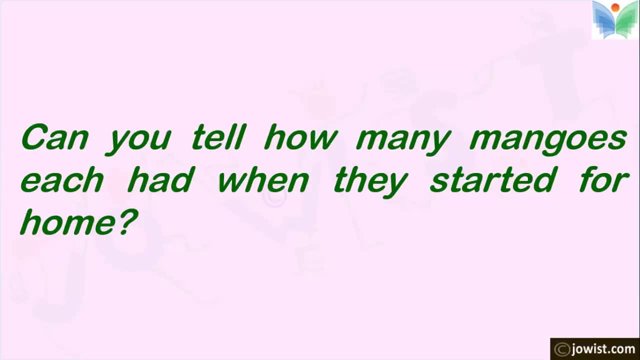 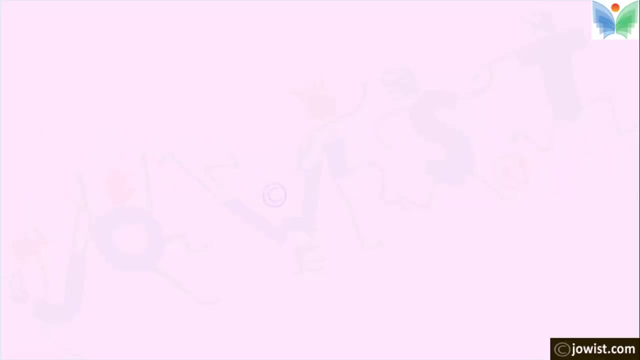 their mangoes. surprisingly, each had equal number of mangoes. Can you tell how many mangoes each had when they started for home? Okay, let us find out. The most important is to make an equation with one variable. If we are successful in making an equation, we are done, Isn't it? What do we know We? 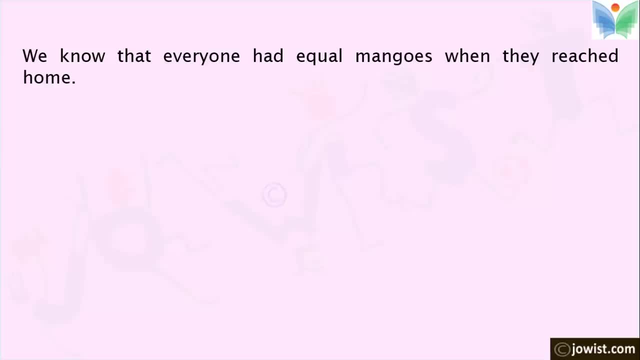 know that everyone had equal number of mangoes when they reached home. First of all, we will make assumption with unknown quantities. Let's assume that when they started for home they had equal number of mangoes, So they had equal number of mangoes when they reached. 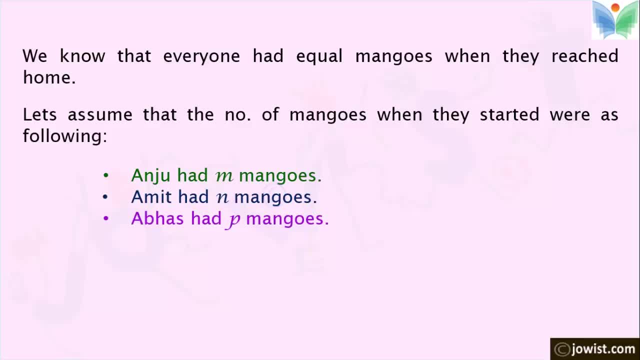 home: Anju had M mangoes, Amit had N mangoes and Abhas had P mangoes. Also, it is given that when they reached home everyone had equal number of mangoes, Say X. On one side there are three variables and on the other side we have single variable which can be related. 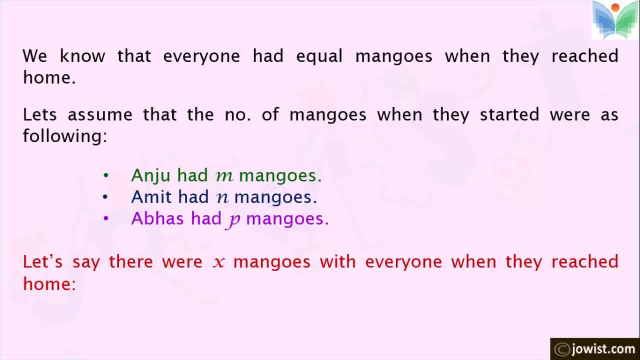 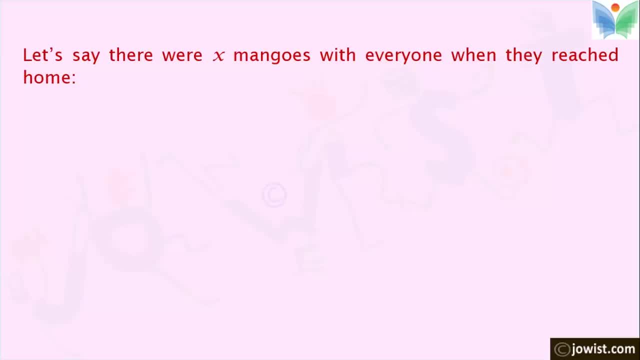 to all three variables. This would be the best place to start towards preparing the equation. Let's also revise facts. It is given that on the way, Anju picked 8 more mangoes, We have also assumed that when Anju reached home she had X mangoes, which also includes 8 mangoes. 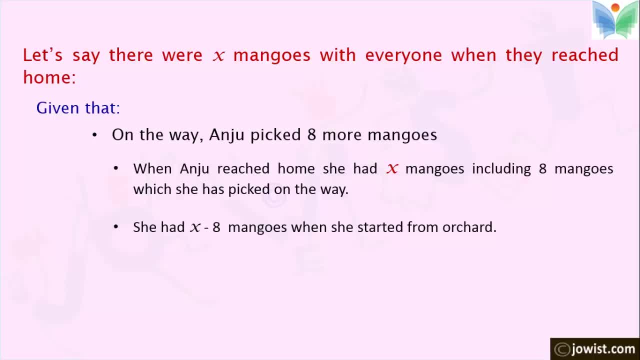 which she picked on the way. Hence she had X-8 mangoes when she started from orchard. Therefore we can say X-8 mangoes. therefore we can say m is equal to x minus 8.. Similarly, Amit ate 4 mangoes from his bag. 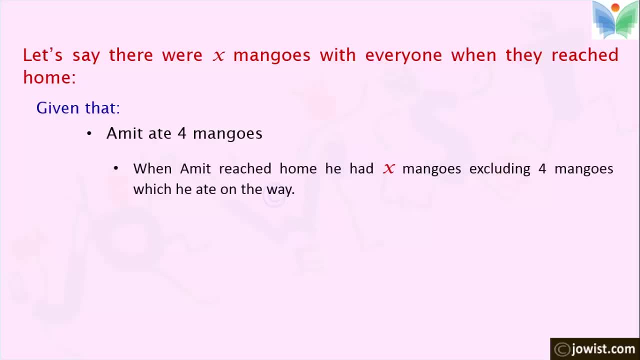 When Amit reached home he had x mangoes. So when Amit started from orchard he must have x plus 4 mangoes. To make it very clear: out of x plus 4 mangoes he ate 4 mangoes and left x mangoes. Therefore his equation will be: m is equal to x plus 4.. As Abhas didn't notice, 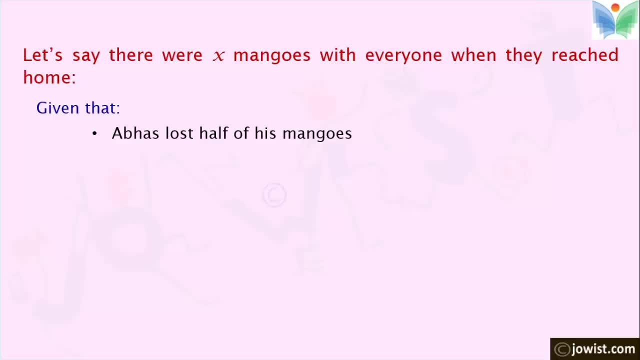 that his bag was stoned, he lost half of his mangoes. When he reached home, he had x mangoes, Hence he had 2x mangoes when he started. In other words, he lost half of 2x and lost half of 2x.